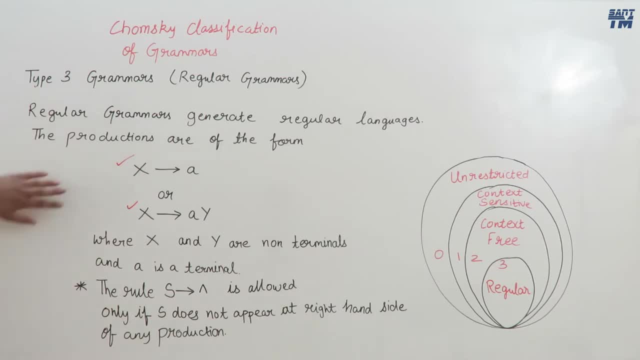 non-terminals and a is a terminal. All the production rules that we have studied till now were of these kind only There is one rule, the rule s derived: null is allowed only if s does not appear at right hand side of any production. What does this mean? 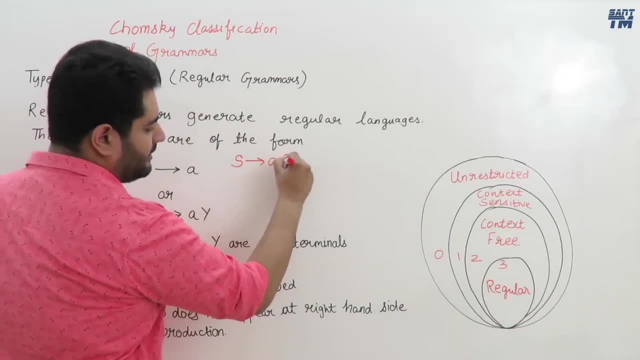 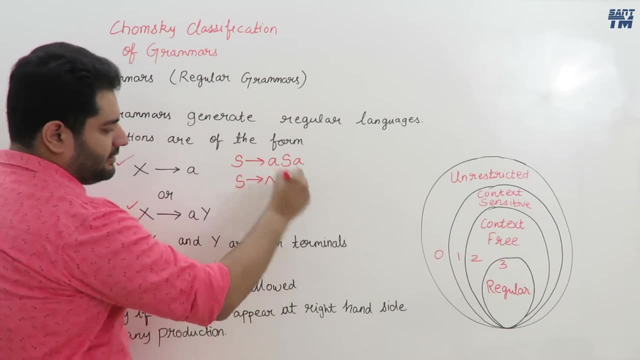 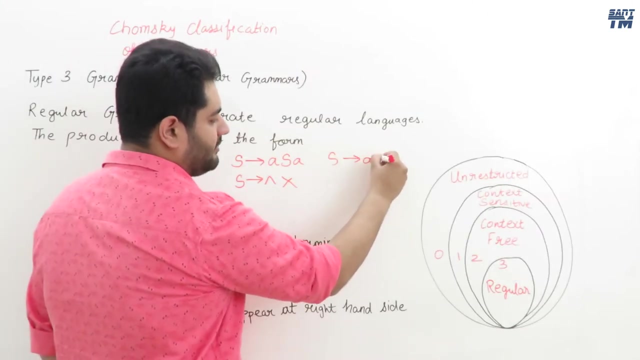 Suppose there is a production s derives a, s a- We have studied many productions like this- Then we cannot use a production rule like s derives null. This is wrong. But if s does not appear on the right hand side of any production, suppose this is the production rule: s derives small, a and capital. 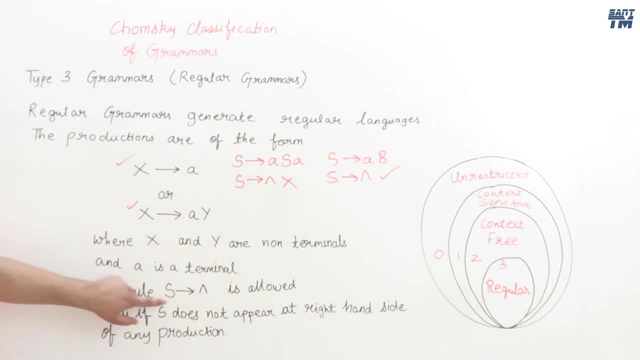 a no it. thank you because it is written. s derives. null is allowed only if s does not appear at the right hand side of any of the productions. see all the production rule In. if any case s is appearing on the righthand side, then you have to remove. 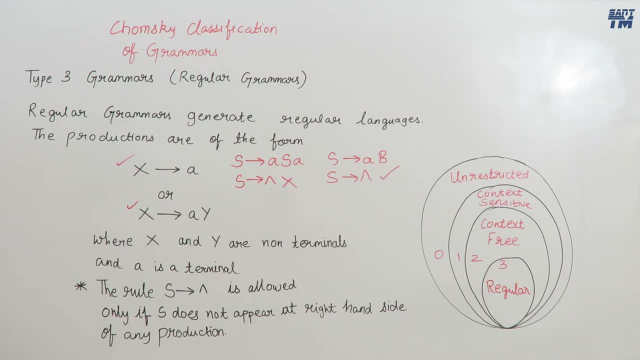 this kind of production. These were the type 3 grammars. Note this rule in your notebook's. Here I have two examples which I can Tibetan scissor. then I will use them in various databases as they seem to have error85 dumplings. 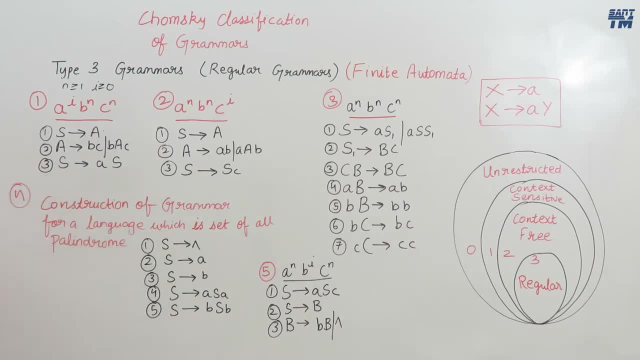 Now, in my previous video you have studied these five examples in which we had to locate a beautifully developed. we had to derive the grammar for a given language. Now we have to test whether they are regular or not. Suppose this was one example: a, i, b, n, c, n in which n was greater than equal. 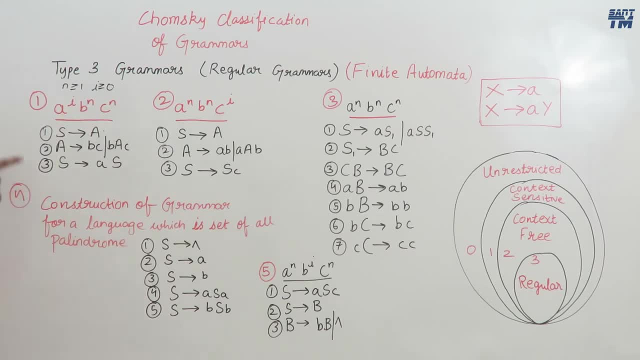 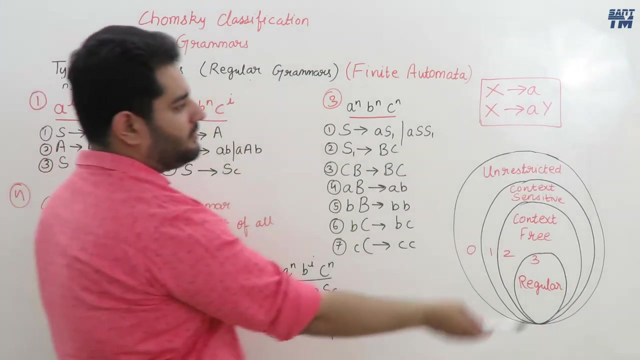 to 1 and i was greater than equal to 0.. So we built up these three production rules for this language. Now we have to check whether it is regular or not. So this production is s derives a non-terminal. a See for a regular grammar. the production rules must be of the. 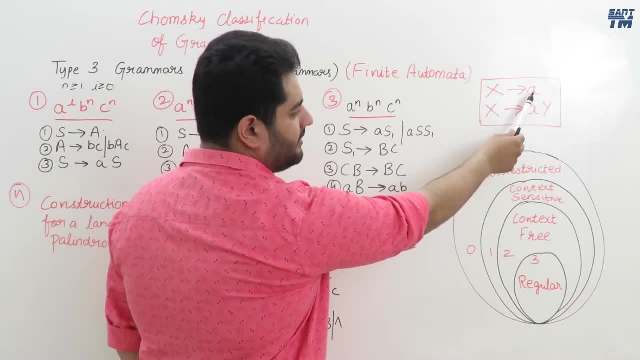 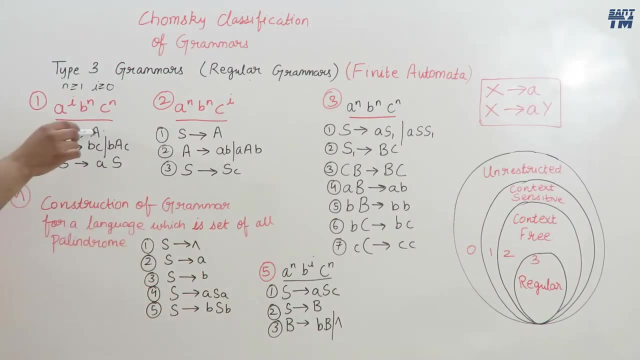 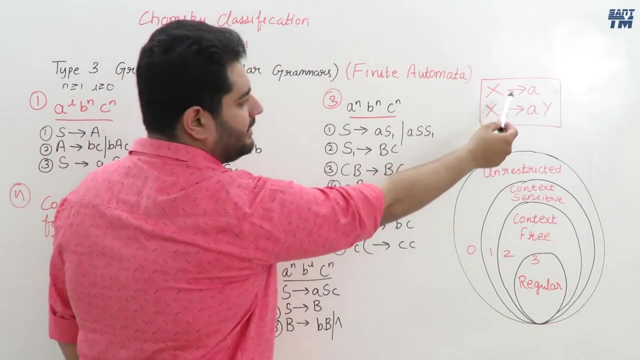 type: non-terminal derives a terminal, and non-terminal derives a terminal, and then followed by a non-terminal again. So s derives a. this is a non-terminal a, But in the case of rules there is no non-terminal. If there exists a non-terminal, then it should be preceded by a terminal. 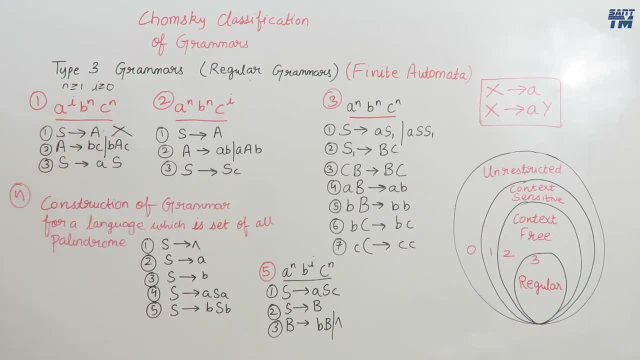 Subtitles by the Amaraorg community. So this production does not follow the rules of a regular grammar. Therefore, we can say that the grammar that we have generated for this language is not regular. Now check for this: a, n, b, n, c, i, s derives a. Again same type of production. So due to this production, 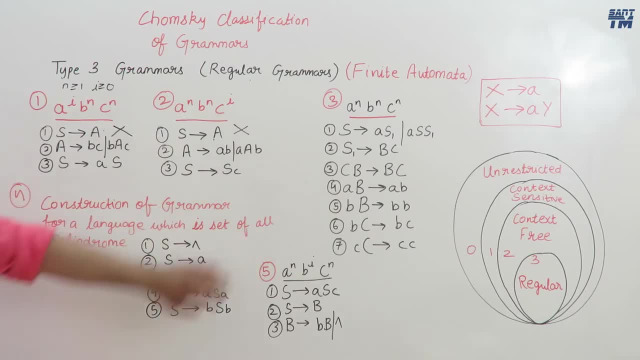 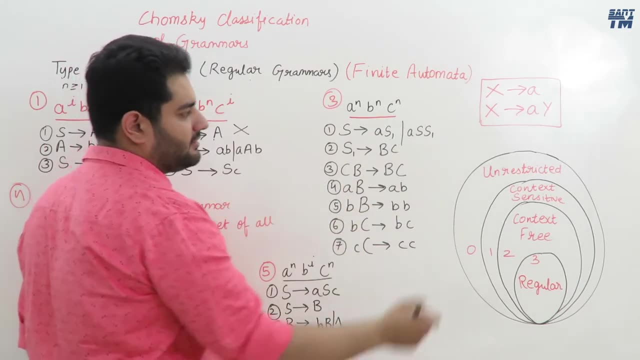 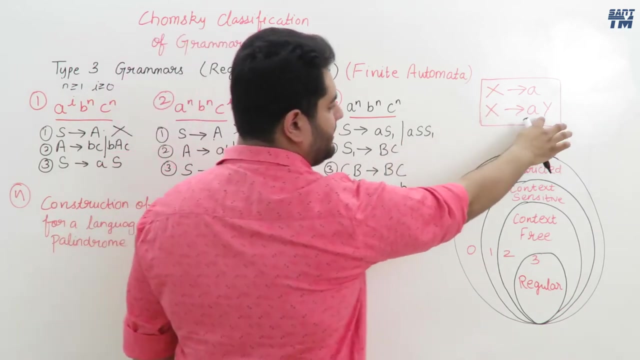 rule. the grammar for this language is also not regular. Now a, n, b, n, c, n. See, here we have s derives, a, Subtitles by the Amaraorg community. Then we have a s s1.. This is also not following this, because we can have only a one non-terminal. 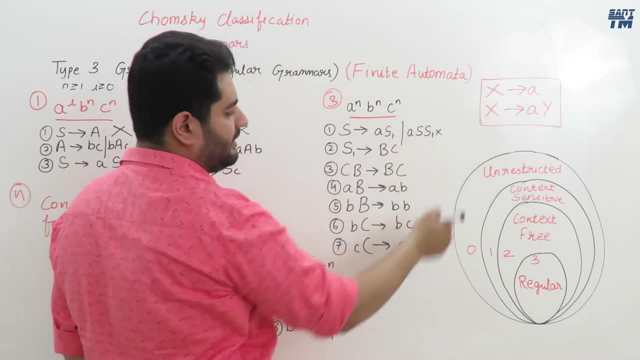 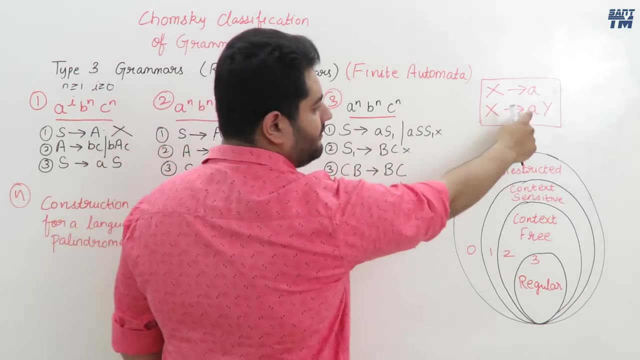 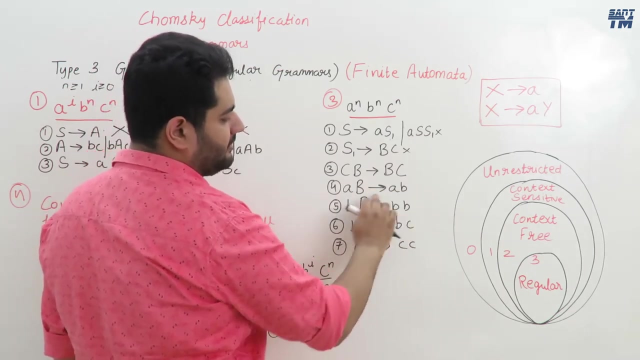 but here we have two non-terminals, So this production is not valid. Similarly, this one is also not valid where s1 derives b c. Both are non-terminals. There should be one terminal at least. c b derives b c is also not possible. and this one is also not possible, This one. 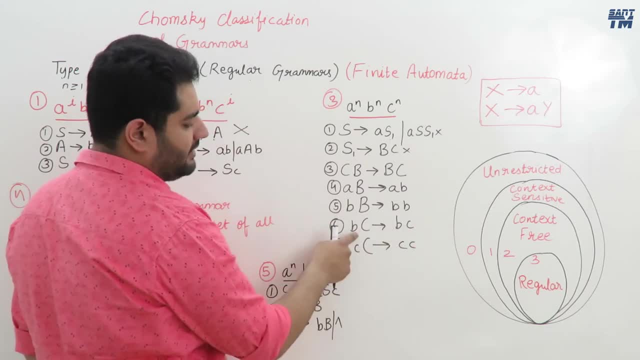 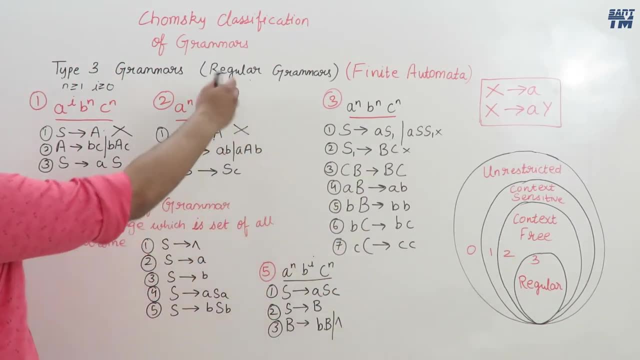 is also not possible. b c derives b c because here should have only one non-terminal. So there are many production rules in this which are not following the properties of normal grammar. Therefore a, n, b, n, c, n will not be a regular language. Therefore not be a. 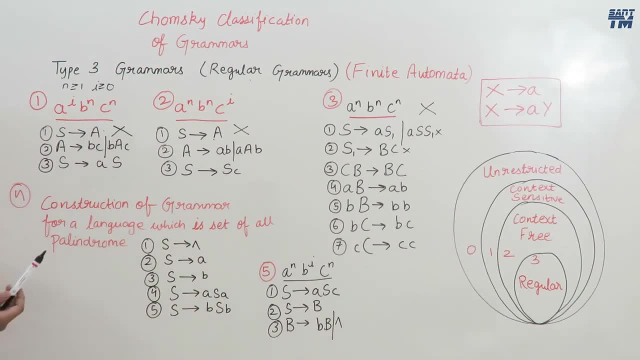 regular grammar. Now there was one question: construction of grammar for a language which is a set of all palindromes. So we built up these five production rules: Palindrome over a, b. There we go. We have a, s n, b, c, i, i, s a n, b, a, n, b, c, a n, b, a n, b, c, i n, b. 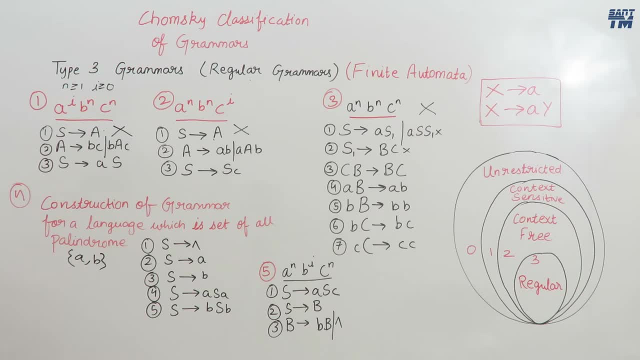 comma B. so here we can see that this production is okay. this is okay. then we have S derived ASA. if we had only AS, then it should be correct. but now we have a terminal, non terminal and then again a terminal. so this is of no kind of to the rule. so this is not valid. similarly, BSB is also not valid, so this: 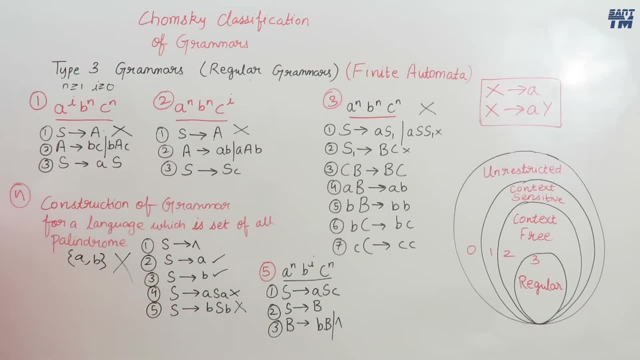 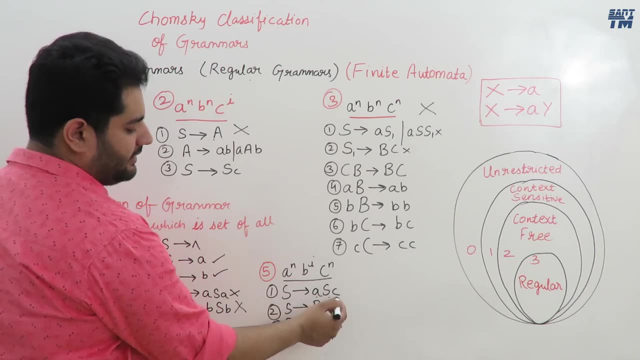 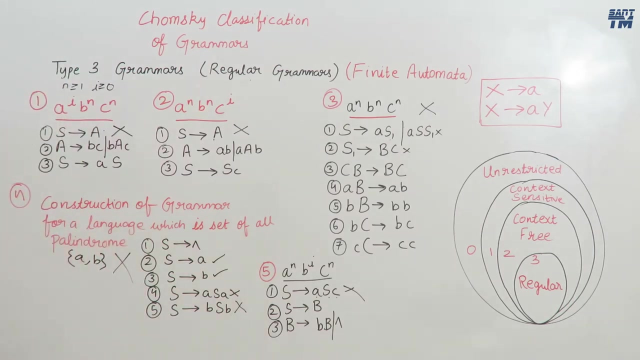 is also not a regular grammar. now here we have AN BICN. this is terminal, a non-terminal terminal, So this is also not following the rules. So a-n-b-i-c-n is also not a regular grammar. Therefore, we can conclude that in my previous videos where I took these 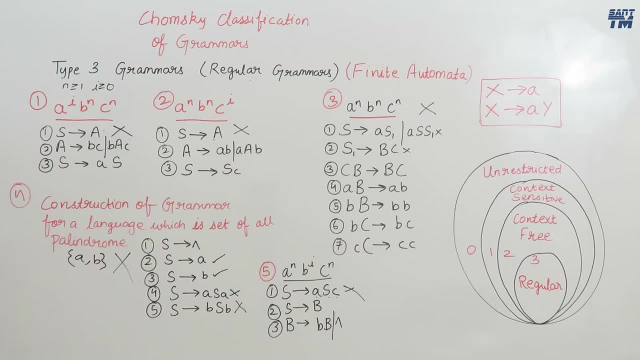 five examples- all those examples for which we have generated the grammar- were not regular. Then we can see, after studying type 2, type 1 and type 0, to which category they belong. So by the time we can say that they are not regular. I hope it is clear to you. And one more thing. 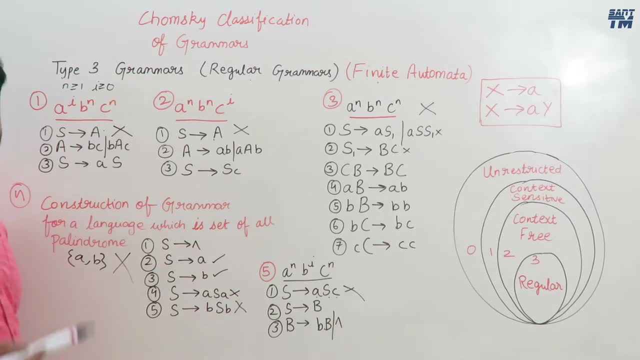 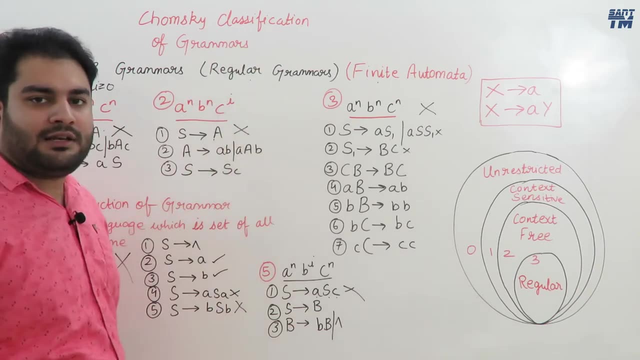 if we have a finite automata for a language- there exists a finite automata or we can build a finite automata for a language- then we can say that that language is regular and the grammar for that language will be regular grammar. This is the property of regular grammar. There must 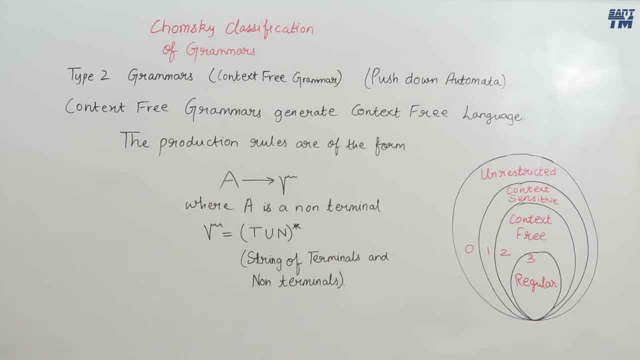 exist a finite automata. Now let's discuss the type 2 grammars, type 1 and type 0.. Type 2 grammars are called context-free grammars. As in the case of regular grammars, finite automata was associated with regular grammar. Here, push-down automata is associated with. 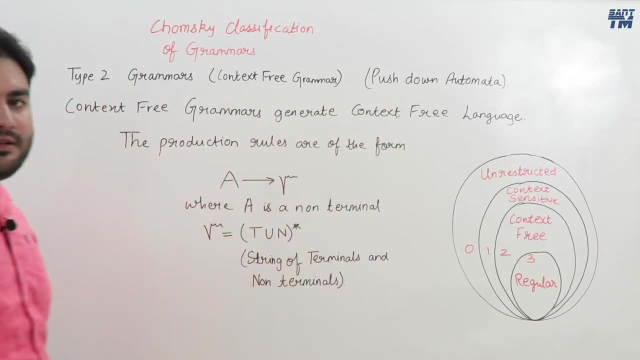 context-free grammars. Push-down automata is also a machine in the subject that we will study later on. Context-free grammars generate context-free languages And the production rules in the case of context-free grammars are of this kind. a derives gamma where a is any non-terminal. 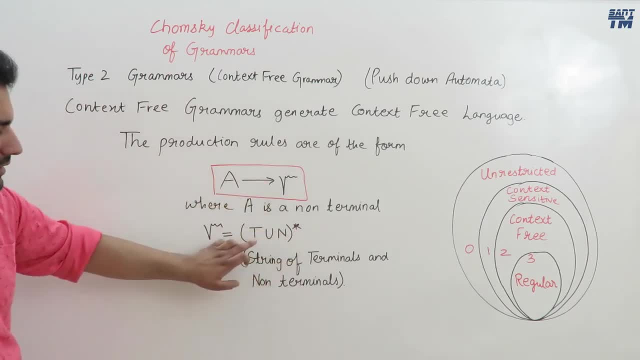 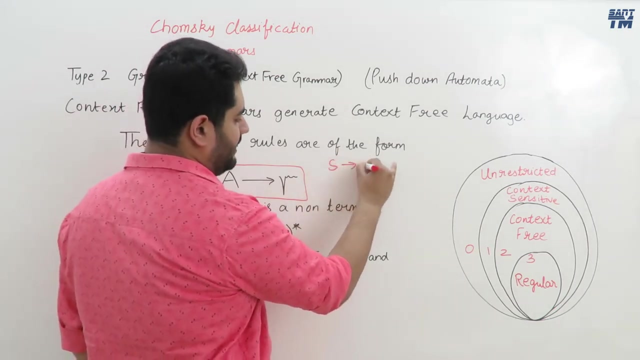 and gamma is a closure of union of terminals and non-terminals. In simple language we can say: any combination of terminals and non-terminals is allied on the right-hand side of the production. Suppose we have a production like S derives ASC, then it is a combination of terminals and 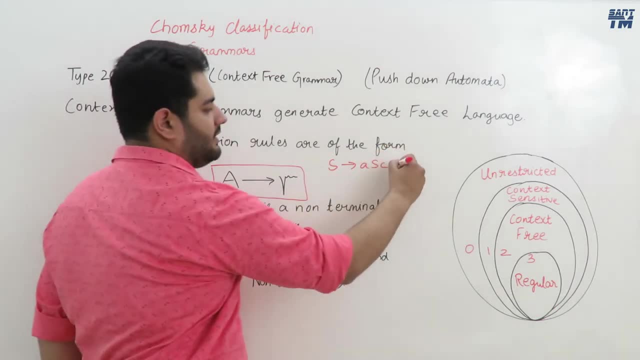 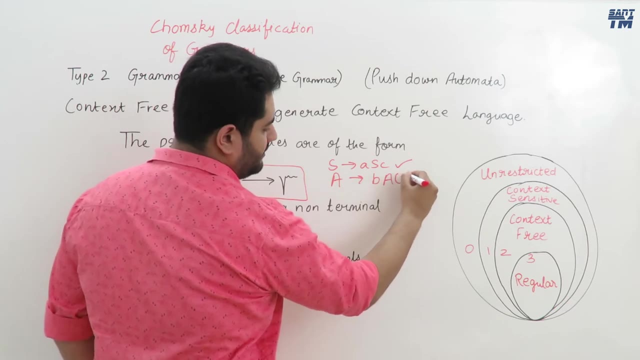 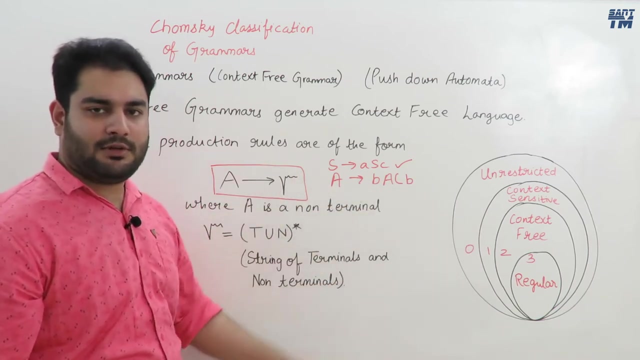 non-terminals on the right-hand side. Therefore, it is in accordance with context-free grammars Or we can have A derives BA. This is also a combination of terminals and non-terminals. Any combination, any possible combination of terminals and non-terminals is allowed in the case of right-hand side. 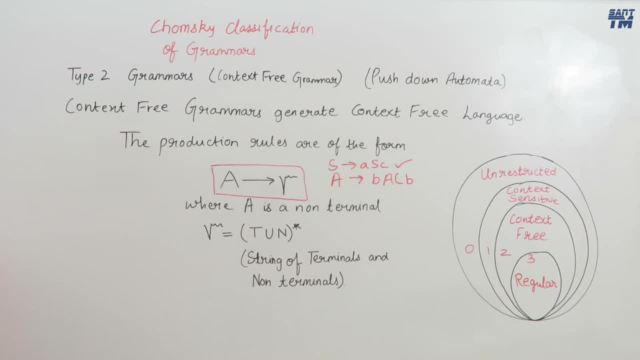 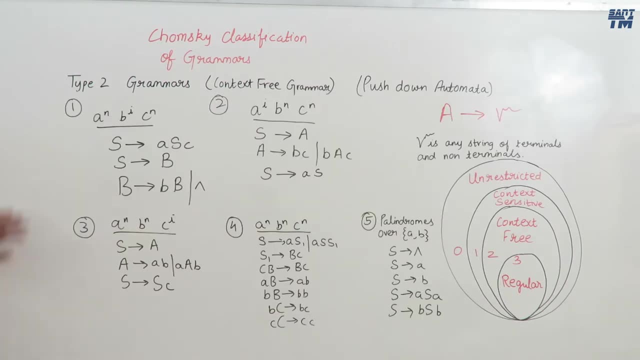 in context-free grammars. So this is type-2 grammars. Now we will discuss the examples, if they are in accordance with type-2 grammars or not. Now see this one ANth BICN where N is greater than equal to 1.. 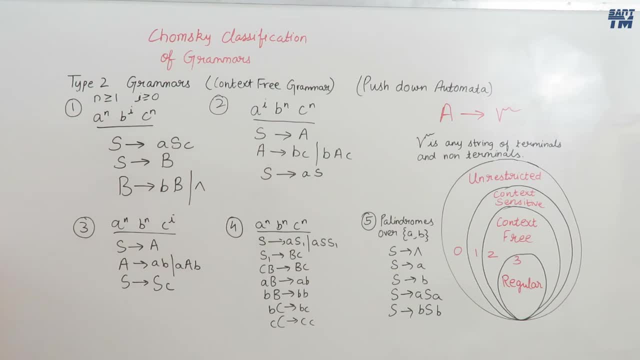 And I is greater than equal to 0.. We built up a grammar for this and we had these three production rules in that. Now we have to verify if they are of type-2 or not. We have already verified that all of these five examples were not regular grammars. Now we are checking. 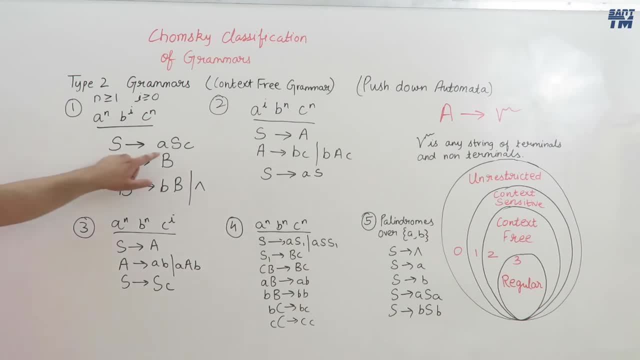 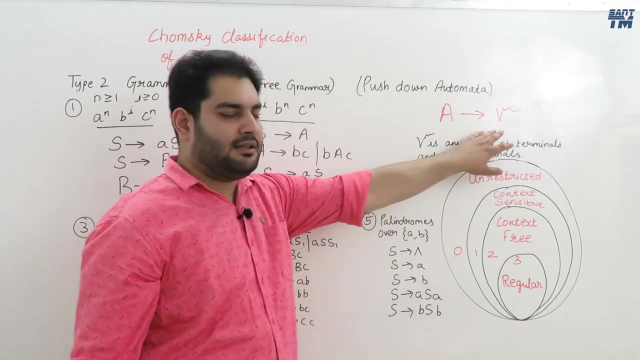 for context-free grammars. So S derives ASC. See this start symbol. S is a non-terminal where A is a non-terminal according to the production. Then it derives ASC. Now in the rule it is said that there must be a gamma such that 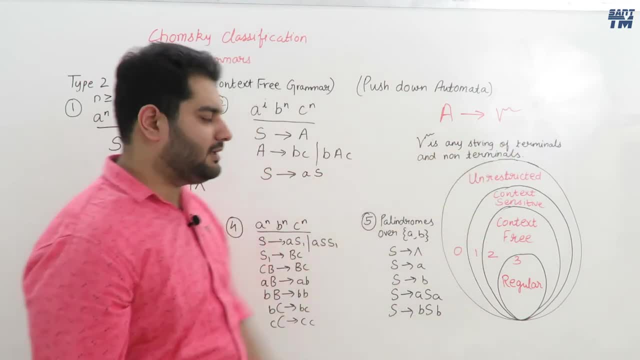 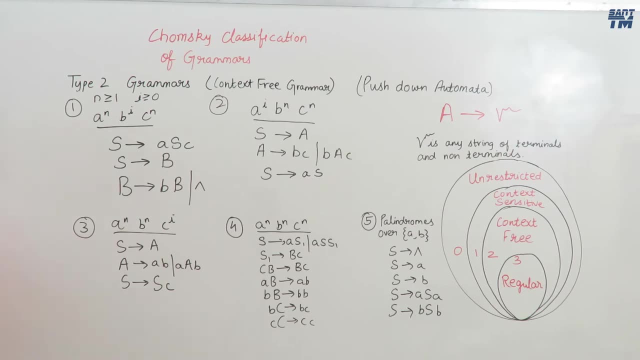 gamma is a combination of any terminals and non-terminals. Here terminal, non-terminal, terminal, That means it is a perfect combination of terminals and non-terminals. So this rule is correct: S derives B. S derives B means it is a non-terminal, and here also we have a non-terminal. So 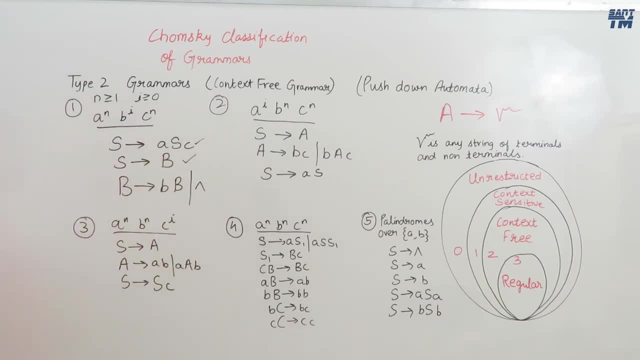 it is also correct. ANTH BICN can exist or even not exist. terminal non terminal B derives terminal B, non terminal B or null. this is also a valid rule because it is also a combination of terminals and non terminal. so that means a NBI CN is a type 2 grammar or. 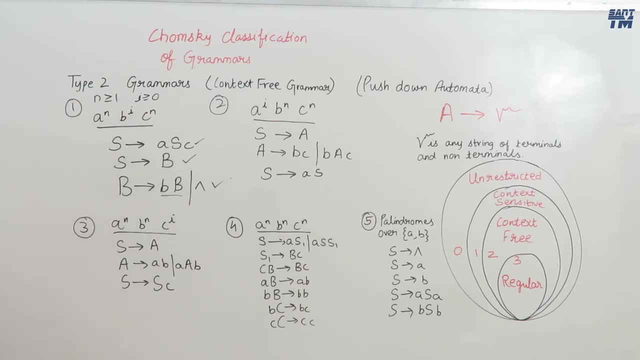 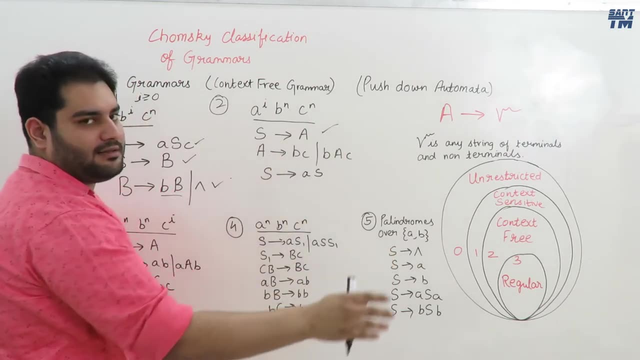 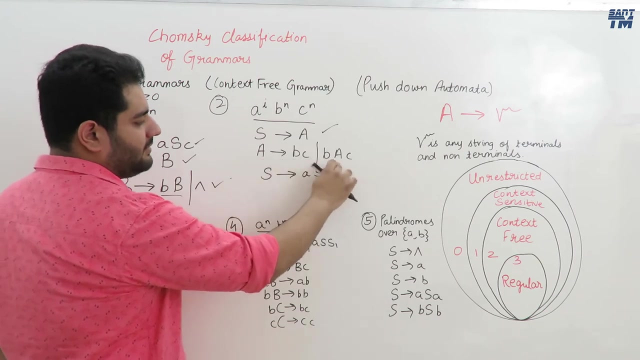 context-free grammar. it is not regular, it is context-free grammar. a, I, B and CN s derives a. it is valid because here we can have anything: combination of terminal or non terminal, either a terminal or either a non terminal. a derives BC, BSE: combination of terminals and non terminals. S derives: yes, it is. 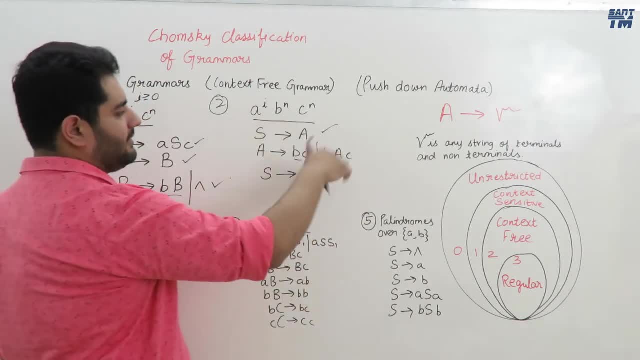 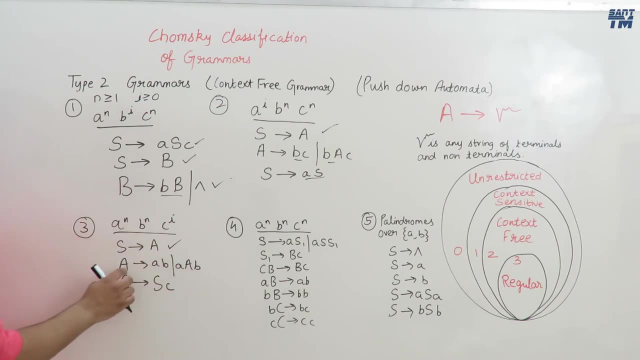 also a combination of terminals and non terminal. therefore, this grammar is also a context-free grammar. a and B and CI. s derives a, it is valid. a derives a, B or a B, it is also valid. s derives sc- it is also valid. all we have is a combination. 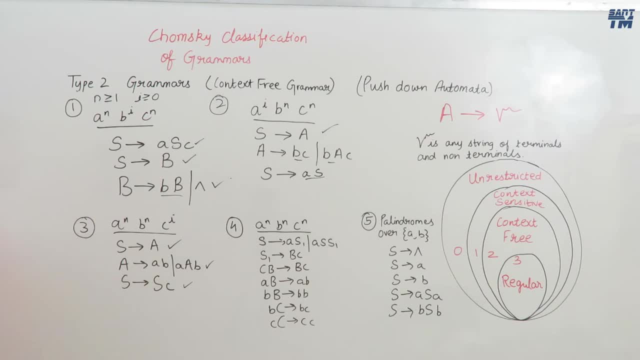 of terminals and non terminals, or either a non-terminal or either a terminal. so this is also a context free grammar. fourth is a, n, b, n, c, n. now note here: this rule is perfect: combination of terminals and non-terminals. combination of terminals and non-terminals. s1 derives, bc is also correct. it is a combination. 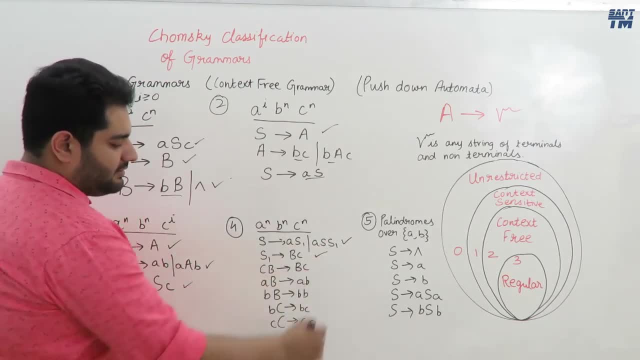 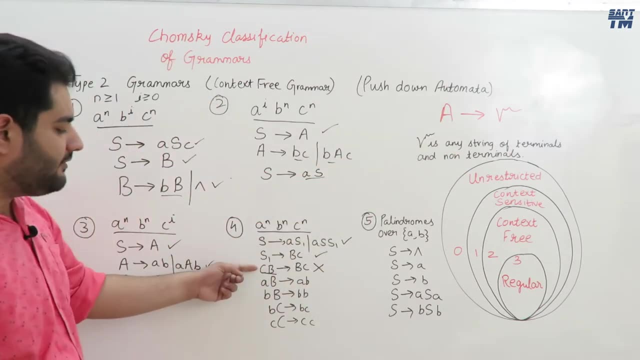 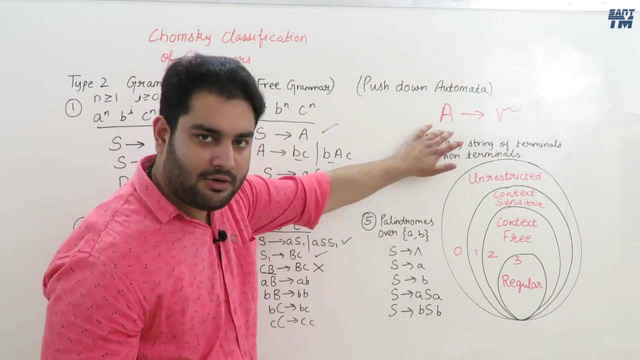 of two non-terminals. cb derives bc. this is not correct. why? because at the left hand side we can have only one non-terminal, but here we have two, and here ab it is having a terminal a and non-terminal b, but we can have only one non-terminal. so all these rules are wrong as per context. free. 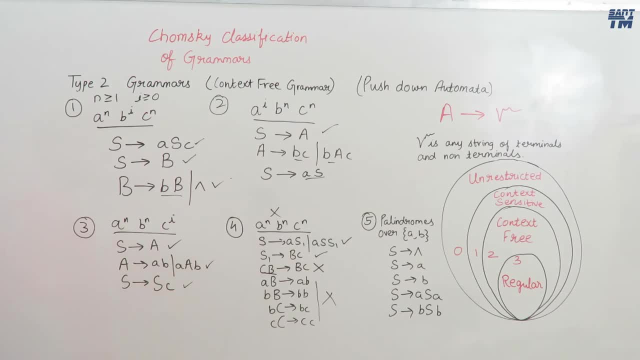 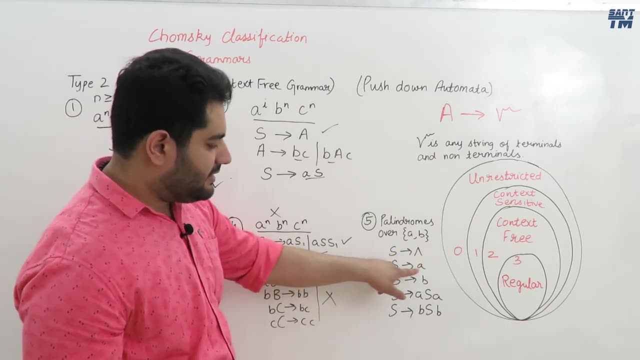 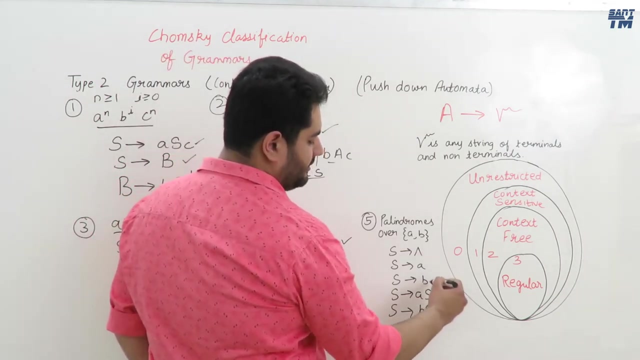 grammar. so a, n, b, n, c, n is not a context free grammar. now one question was palindromes over a and b. we derived these production rule s derives null, s derives a, s derives b, s derive asa s derive bsb. combination of terminal and non-terminal. it is also. it is also correct. it is also correct. it is also correct. 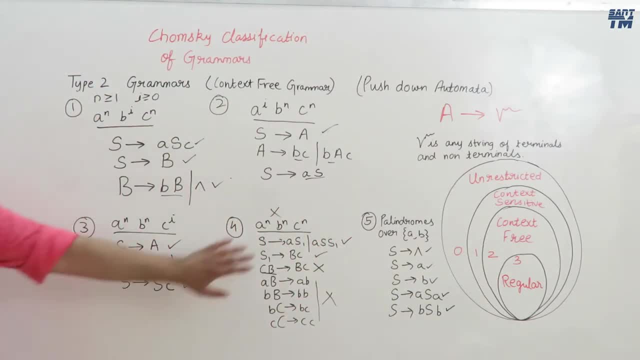 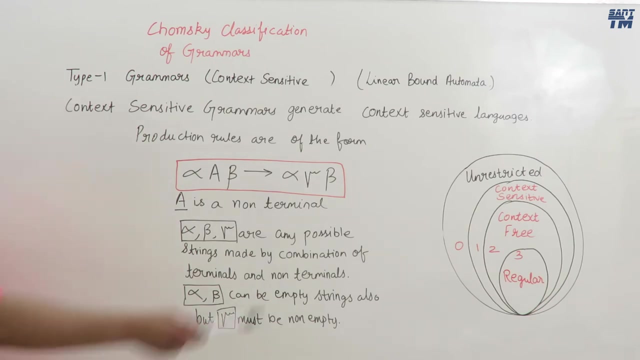 so, out of these five examples, only this one was not context free grammar. rest: all other were context free grammars. now we shall discuss the type one, that is, the context sensitive grammars. now let's discuss the type one grammars. type one grammars are called context sensitive grammars. 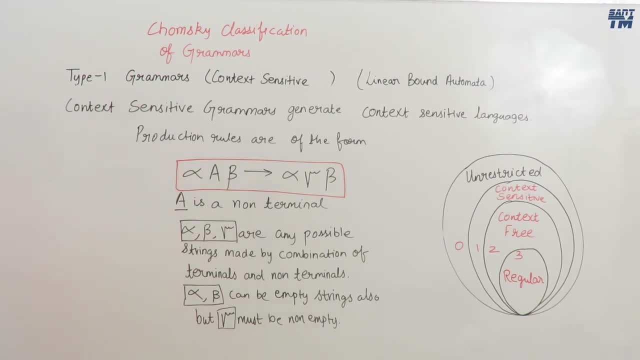 as it was: finite automata for regular languages. push down automata for context free languages. there is linear bound automata for context sensitive languages. out of these, till now we have only studied about finite automata. we will study later on about push down automata and linear bound automata. so context sensitive grammars generate context sensitive. 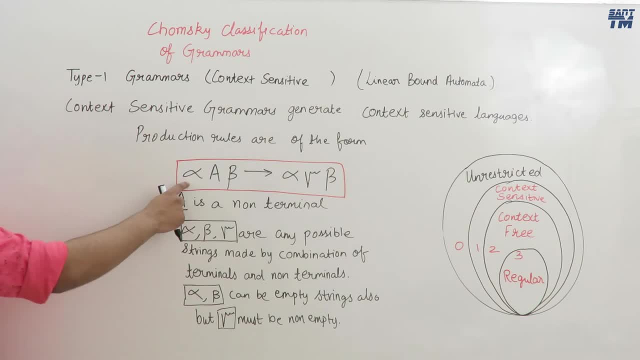 languages. the production rules are of the form alpha. a beta derives alpha, gamma, beta. here only a is the non-terminal alpha. beta and gamma are transform it into a closed form and there is no difference inきn illegion between these terms. alpha is Boolean and comming is a non-terminalento a. 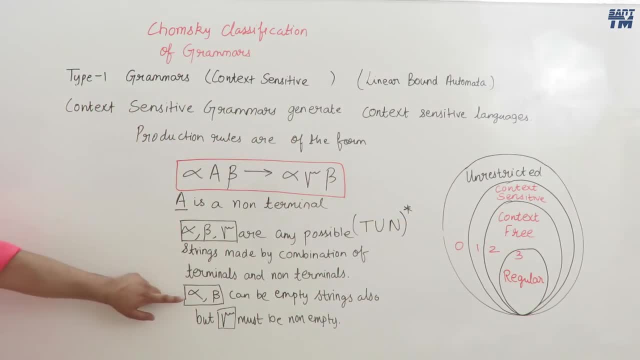 representative of complex geometry of européan Ple. Airbnb is expressed as a phi. that is the cause and theщ of inter quiz is: mean alpha ever as empty. then common talk of alpha as empty and consider α and beta as empty and consideruse a bit. so accidents only. we can leave only it As we need to reduce a bit. lemme show these Kruger equations here and we write down: alpha and beta is empty and considerjing it and to useин ekandaka addition and consider exponents. 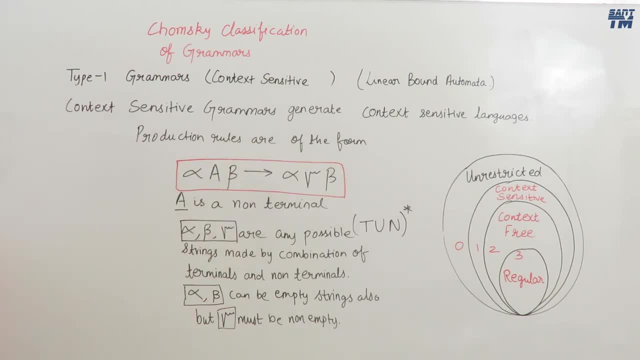 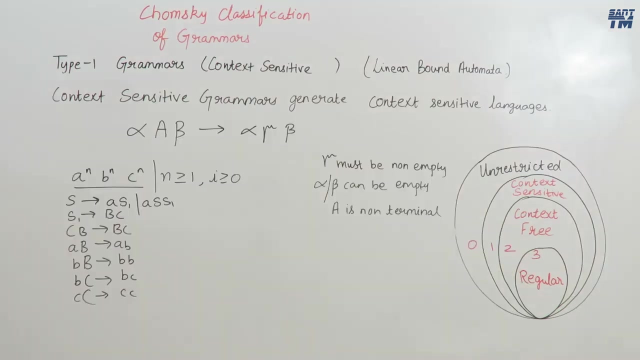 alpha a. so there is no error in that alpha and beta can be empty also, but gamma must be not empty. that is, we cannot leave gamma as a empty string. we have to consider a string for gamma every time. so let's see one example now. consider this example: a, n, b, n, c, n. this was not 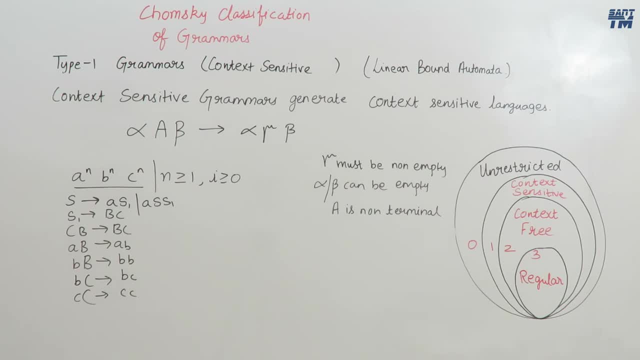 proved to be context free. let rest, other were proved context free. so we are checking it for context sensitive. so these are the production rules and we have to check. if these production rules are of this form, then we can say that it is context sensitive language. so first consider: 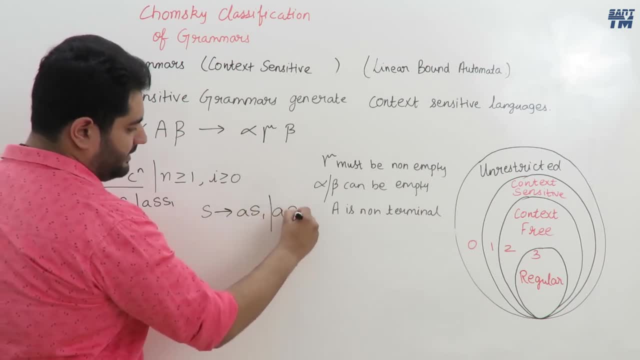 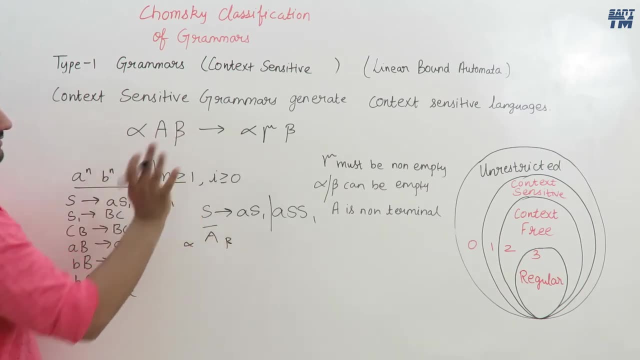 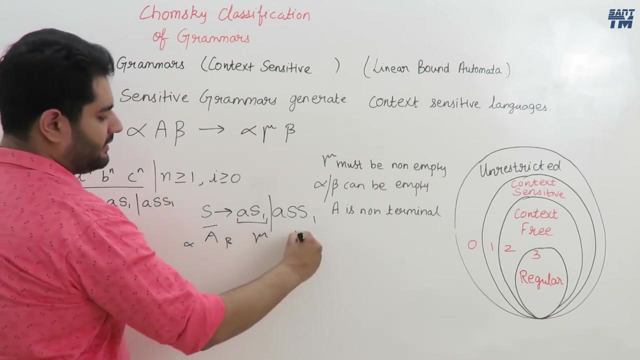 s derives a s 1 or a s s 1, then if we take this s s a, then we can say that alpha and beta are empty for this lhs, then this is: if lhs is having alpha and beta is empty, then it is gamma and this is. 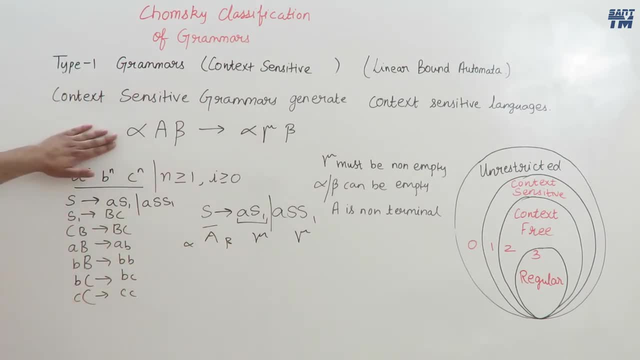 also gamma there. therefore, this is satisfying our production rules. so this is a valid production rule as per context sensitive. now we check for: s 1 derives b c. s 1 derives b c. here, if we take s 1 as a and this as gamma, we can say that alpha and beta are empty. so this is also a. 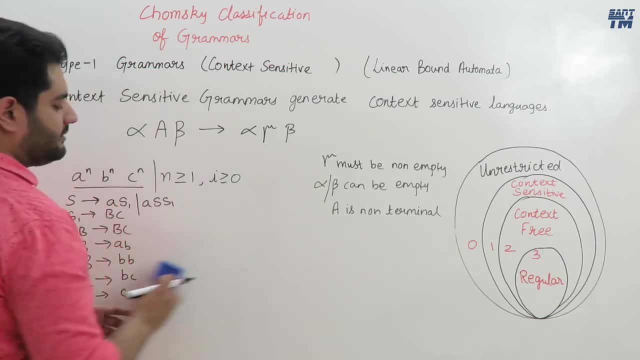 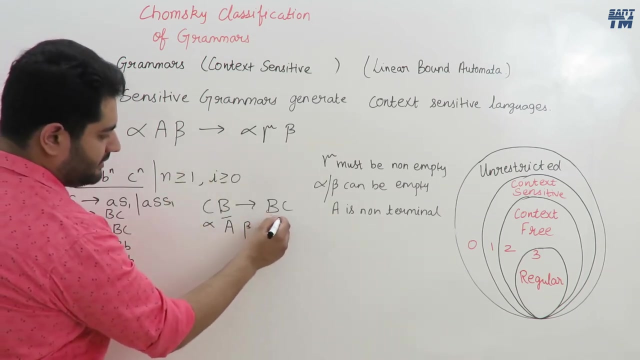 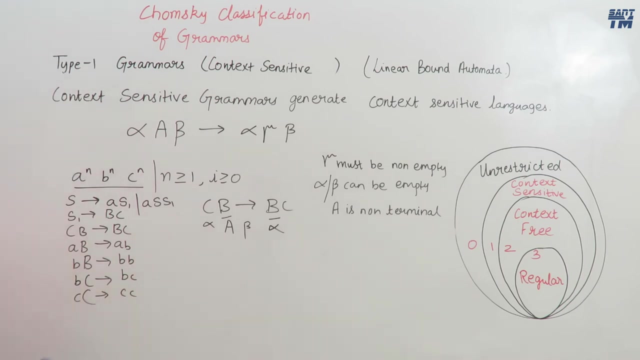 valid production rules. now, c b derives b c, see it very carefully. c b derives b c. and now if we a pause, a pause, see it very carefully. c b derives b c. then if we take this as alpha- and this is also a valid piece- ad a depends on whether this is omega or cb. right in searching. if we look at an exaggerating 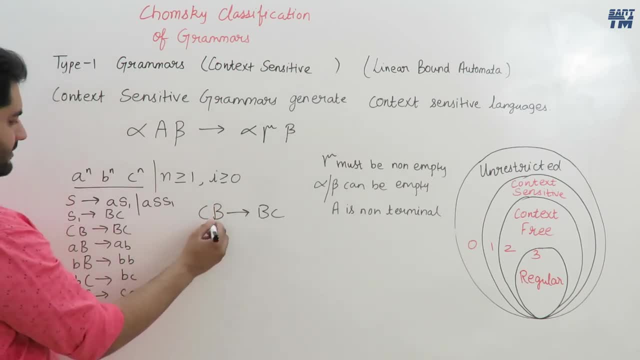 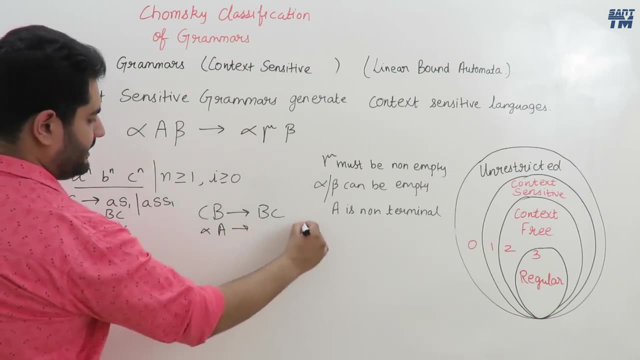 a is not a perfect one, b or c, then 봅 b or cb is alreadyetz andуж cb is alreadyetz duas lleb il lhs soobhi. in the search 구 selective cb derives b, c. then if we take this c as our alpha and b as our a, then beta is empty here. so we have to keep beta as empty here. 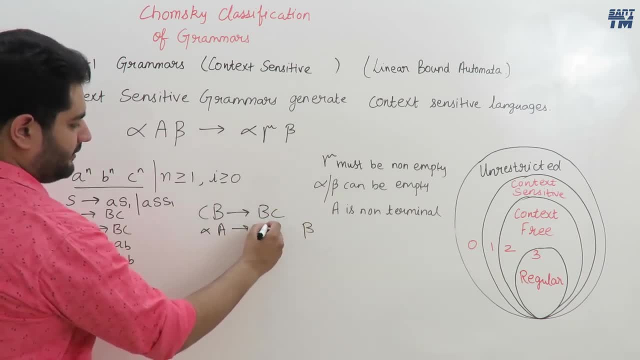 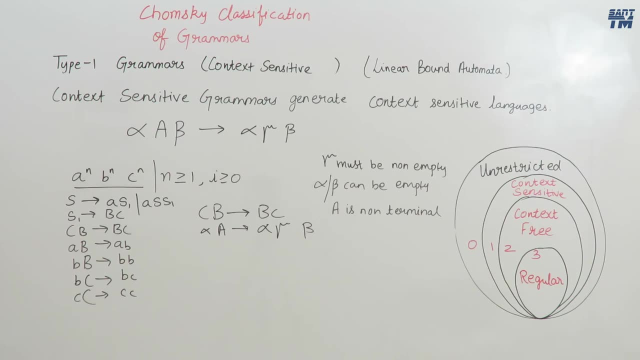 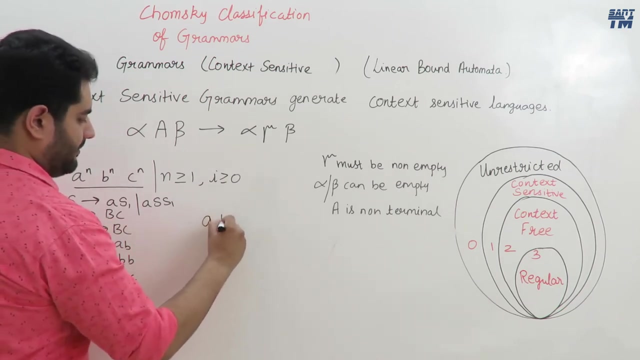 now here we can see that it can be of style alpha gamma, because beta is kept to be empty. so this is also a valid production rule. now check for a capital b derives small a small b. a capital b derives small, a small b. if you take this as alpha and this as a, then you can say that. 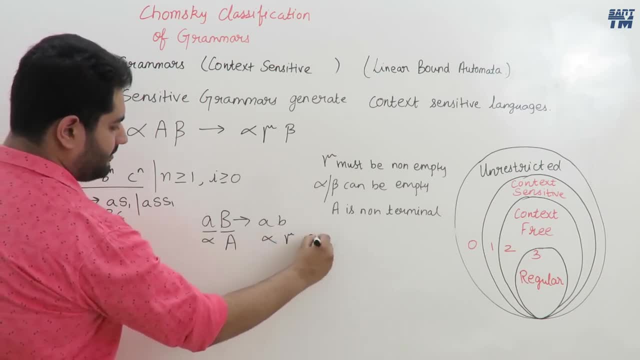 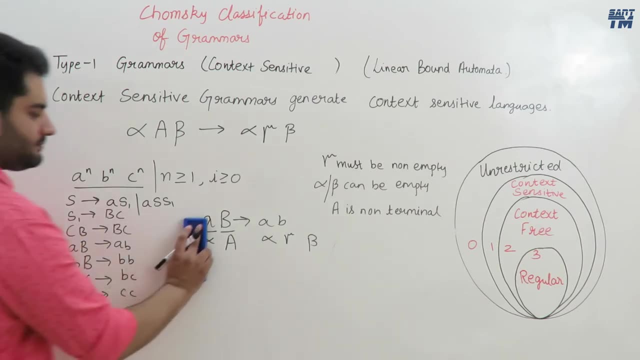 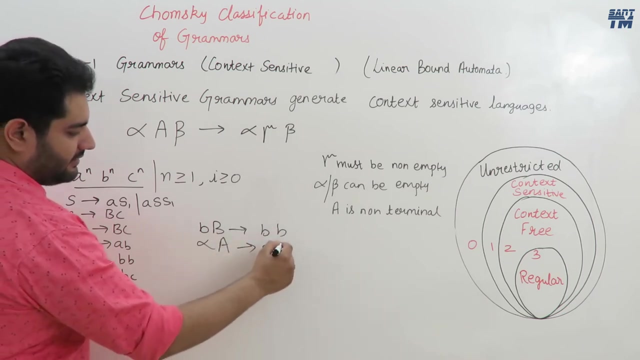 this is alpha, this is gamma, and beta is empty here and beta is empty in the lhs also. so this is also a valid production rule. now check for bb derives bb. if you take this as a, this is alpha and beta is empty here, then you can say that this is alpha, this b is alpha and this b is gamma. and 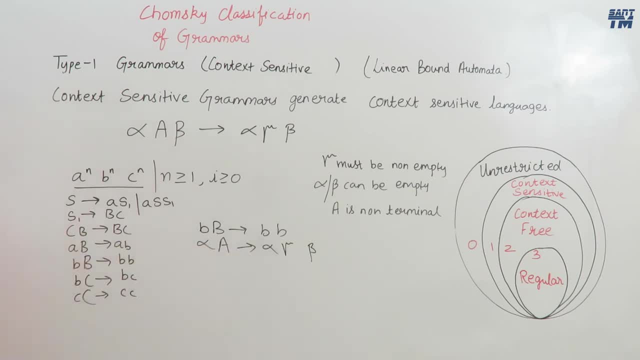 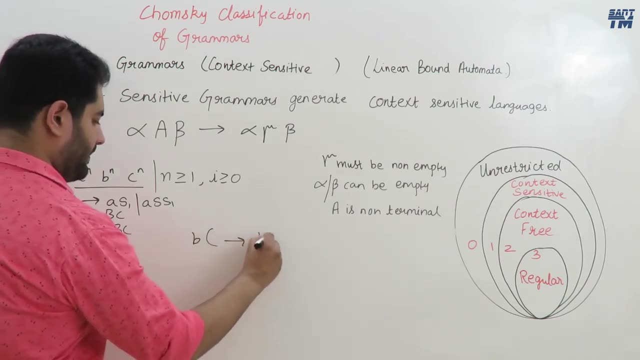 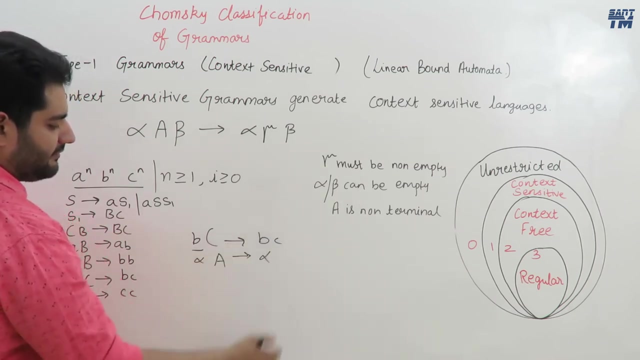 beta is empty here. so both lhs and rhs are having. beta is empty, so this is also a valid production rule. check for bc: if you take this is alpha, this says a and beta is empty. you can say that this b is alpha and this c is gamma and beta is empty here. so this is also a valid production rule. 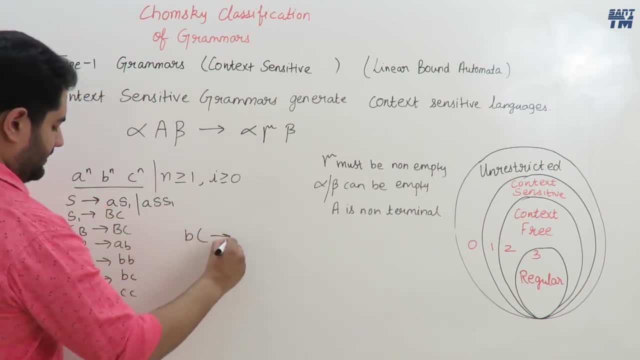 now check for this one. bc derives bc. alpha a. alpha gamma beta is empty. beta is empty here, so this is also a valid production rule. now check for c capital c derives cc. alpha a beta is empty. alpha gamma beta is empty, so this is also a valid production rule. so all the production rules that we have derived for a grammar that. 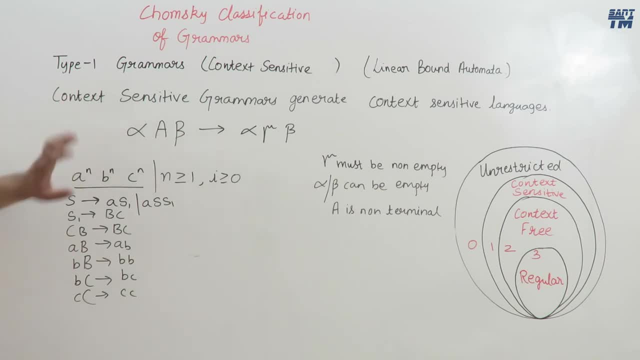 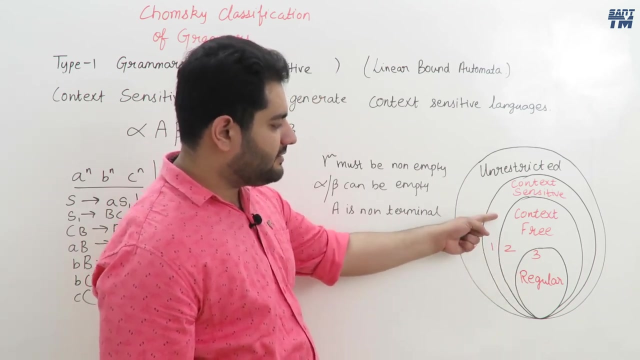 will generate. this language is satisfying this property of context sensitive grammar. so this is a context sensitive grammar. now note that in this hierarchy derived by norm chomsky, he is saying that type 3 is regular, type 2 is context free, type 1 is context sensitive and 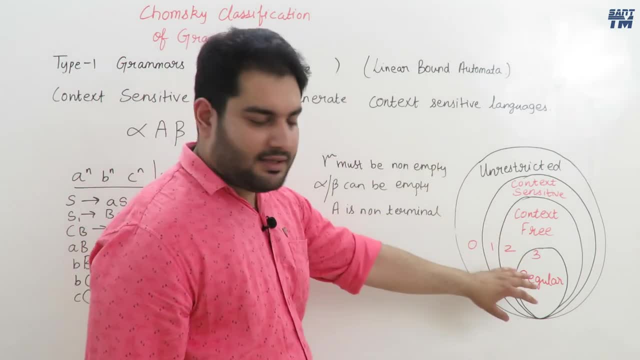 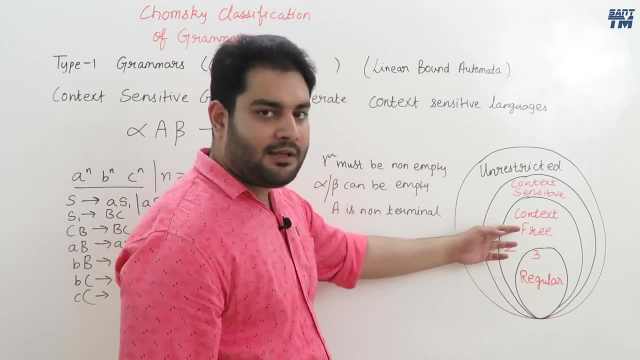 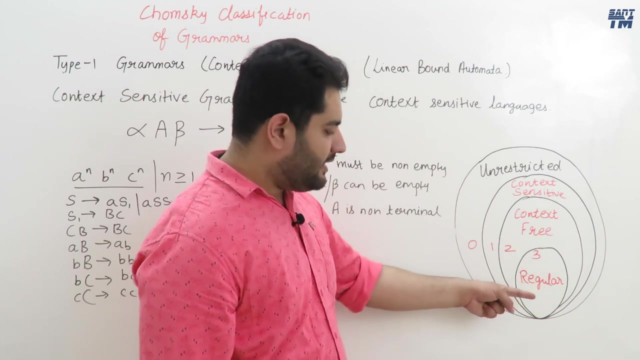 type 0 is unrestricted from this hierarchy. we can say that every regular grammar is context free grammar also, and every context free grammar may not be a regular, but regular grammar is lying inside the block of context free. therefore, we can say that every regular grammar is context free, every context free, context sensitive, every context sensitive. 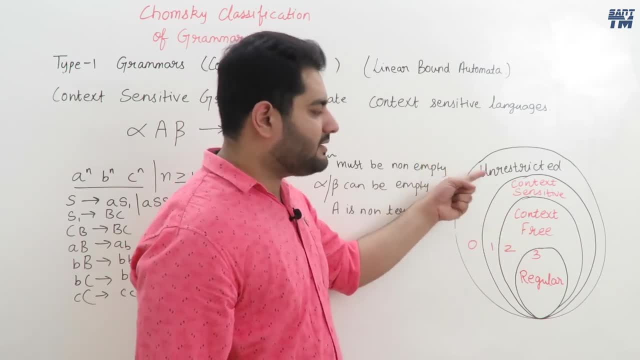 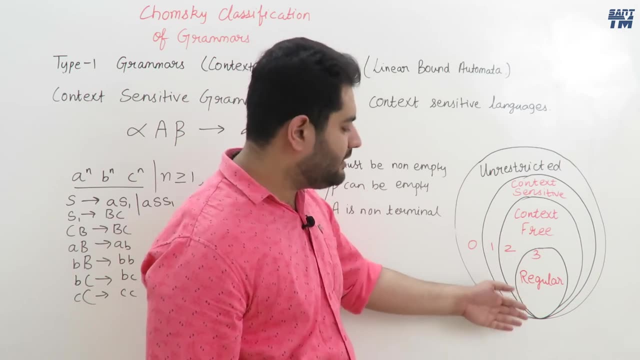 is unrestricted. but it may not be true that every unrestricted is context sensitive, or every context sensitive is context free, or every context free is regular. only we can follow the hierarchy from bottom up. so onlywang to back pass into the next section. if you are interested in the actual context, freeUUU sth your're interested in the lieber athe is whatever, or sth this Umge B на A beother Chomsky. 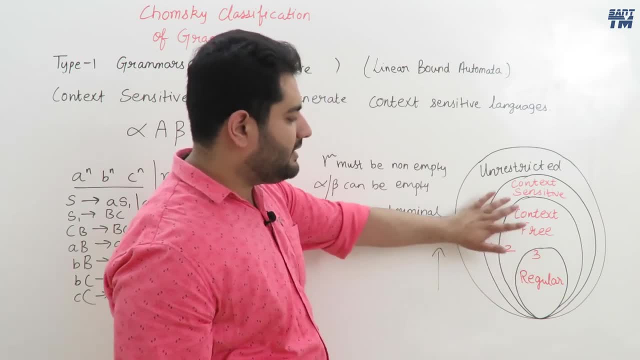 only we can follow the hierarchy from bottom up, come over to the answer. a lot, but for this, context free is context free. managed by the intention to kindling by root is NaK to up. regular can be context-free. context-free is context sensitive and context sensitive is unrestricted. so by here we can say that this example is: 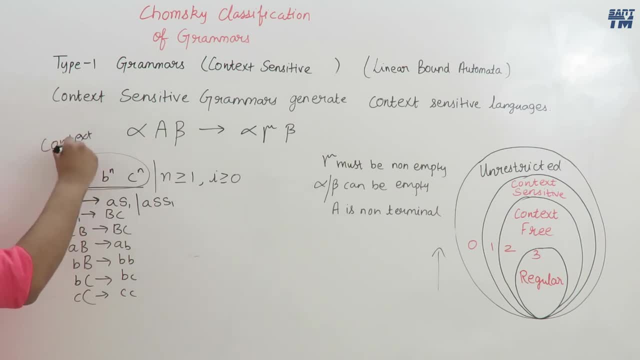 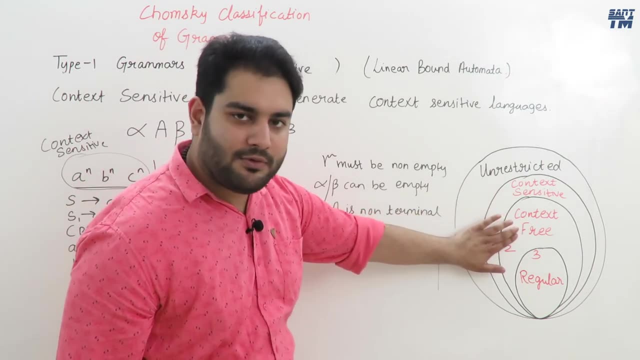 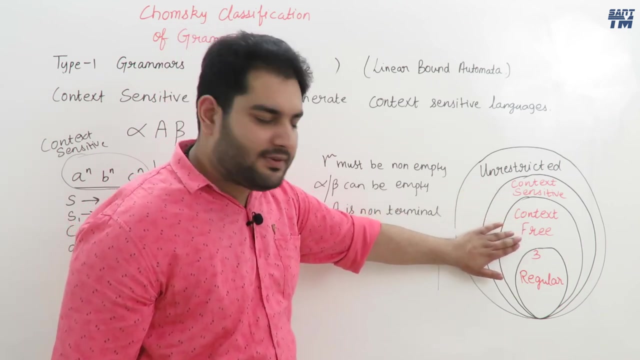 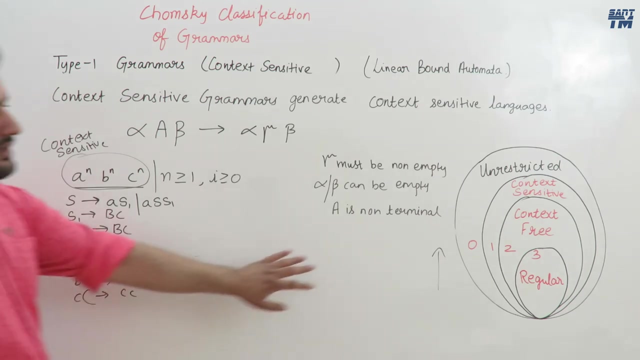 only context sensitive because it was not proved context free. so it is only context sensitive. and all those that were proved context free are also context sensitive, because context sensitive is lying upper in the hierarchy. all the context free are context sensitive. all those four examples are context sensitive also, but this one is lying only in context. 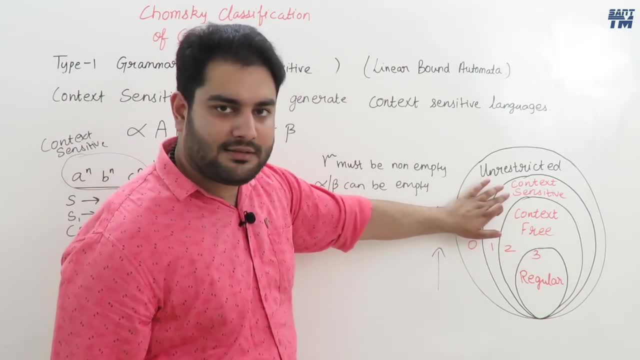 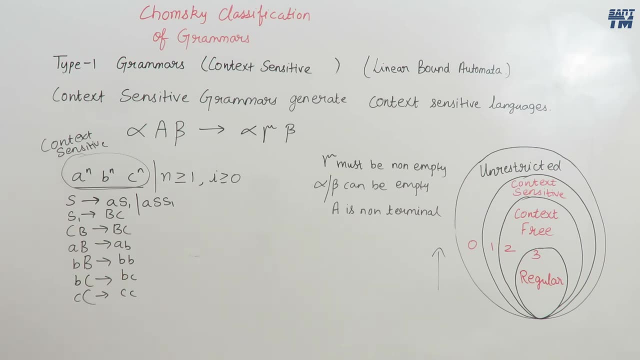 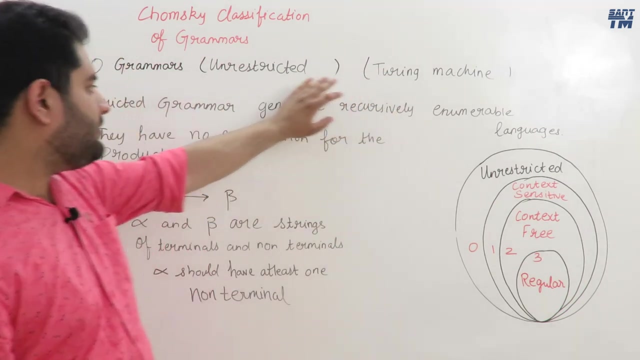 sensitive and not in context free. so this is only context sensitive, not context free. so I hope this is clear to you. now we will discuss the type 0 grammars. now type 0 grammars are called unrestricted grammars. Turing machine is the automata for the unrestricted grammars. unrestricted grammars generate. 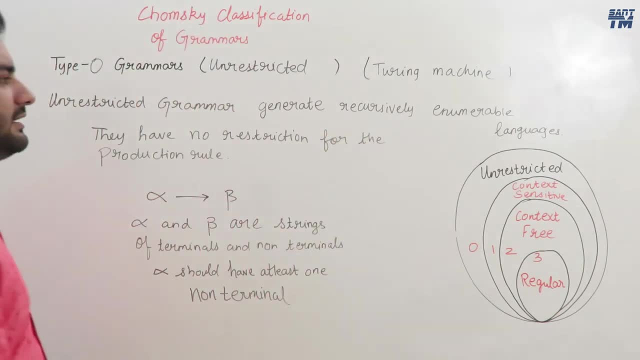 recursively innumerable languages, the name for the language is recursively innumerable for unrestricted grammar. by the names suggests we can say that they have no restriction for the production rule. the production rule can be of any kind. alpha derives beta, where f and beta, both are the combinations of terminals, are non terminals. 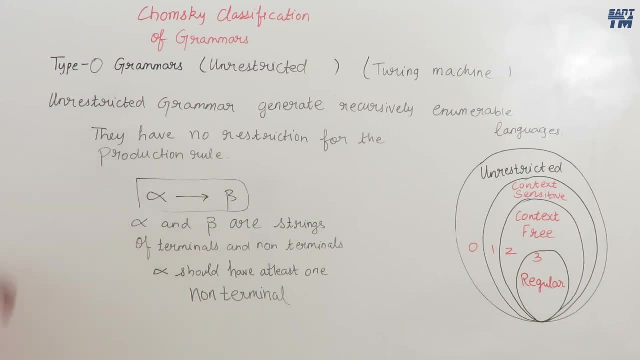 only one specific property exists for this type of grammar and that is alpha. that means the LHS of the production rule should have at least one non non-terminal rest. everything is accepted by this grammar. only one property it specifies that is lhs should contain at least one non-terminal. it is not possible that lhs contains only terminals. 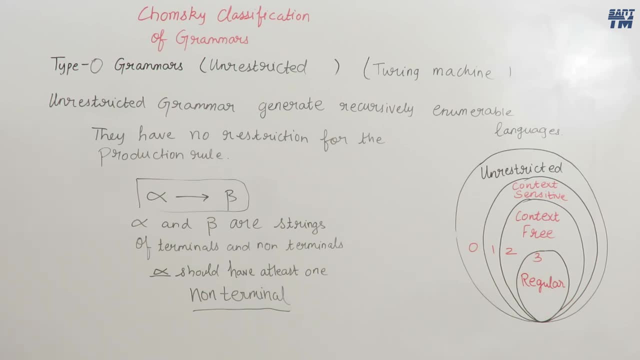 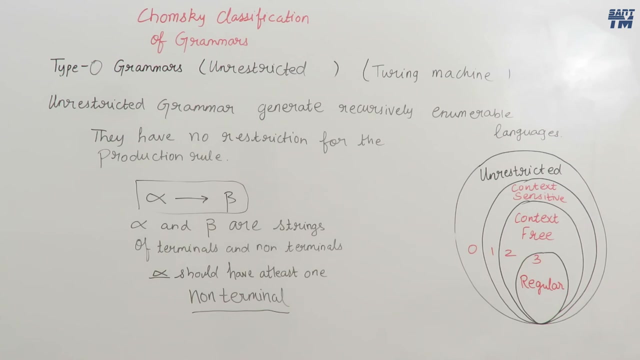 because that production rule cannot be a valid production rule because we cannot replace a terminal, we can only replace a non-terminal. so it is always kept into mind. so finally we can say: all regular languages are context-free languages, all context-free languages are context-sensitive languages, all context-sensitive languages are unrestricted languages or all.